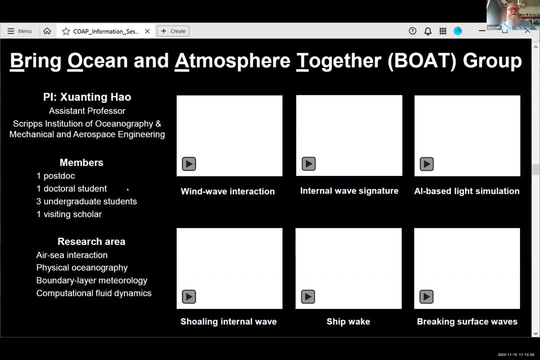 So Professor Howe is a new assistant professor here, joint between scripts and mechanical engineering, looking at different wave interactions, but unfortunately I lost the animations. So Professor Howe is a new assistant professor here, joint between scripts and mechanical engineering, looking at different wave interactions, but unfortunately I lost the animations. 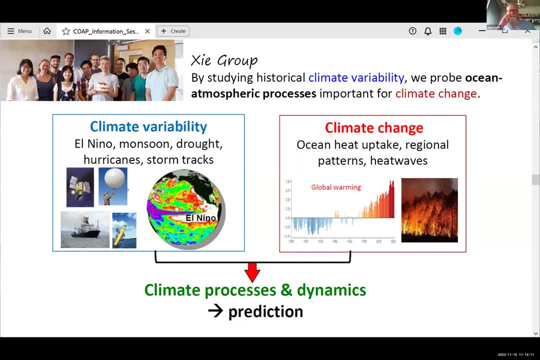 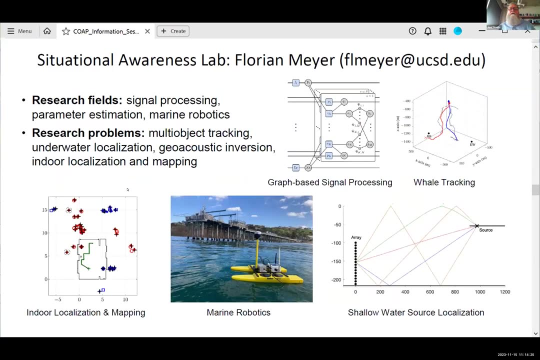 Hongbing Zhui has been looking at climate variability Also to better predict climate change and how climate variability will shift. with that, Florian Meyer is also a relatively new professor here with a lot of work in acoustics. As you see, Florian Meyer is also a relatively new professor here. 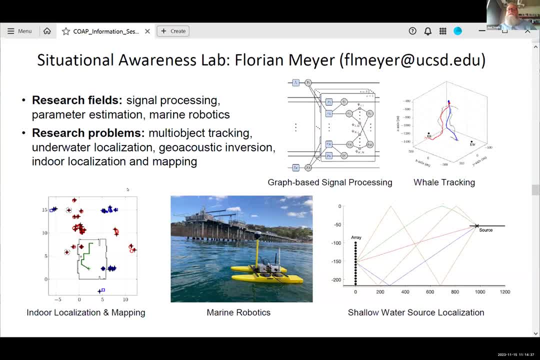 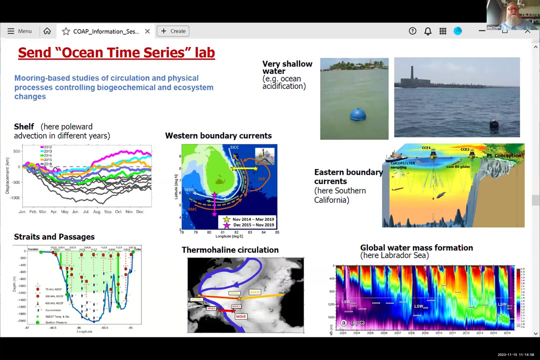 with a lot of work in acoustics that trying to figure out both the whale tracking you can see there but also what can be understood about ocean through acoustic measurements. Huve Sindh is another one of our labs, here Again also with a lot of in situ measurements and gliders. 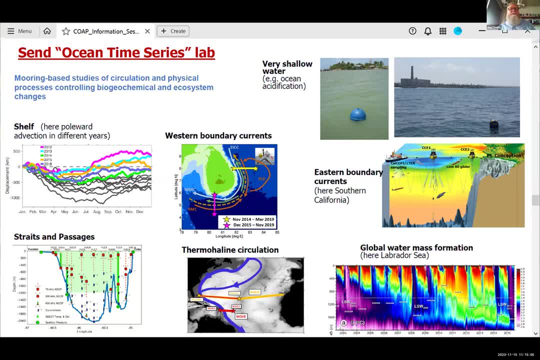 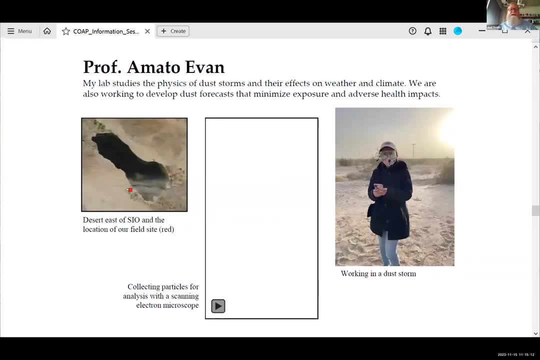 monitoring of processes in the ocean. Professor Amado-Evan is recently getting into dust aerosol, especially in the Salton Sea region, which is east of the mountains in San Diego, trying to understand what develops dust storms and the impacts they have. 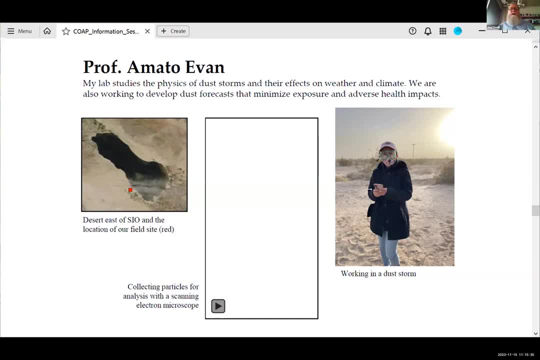 I've showed you some research here. If any of this is interesting, you can contact the professors here. Some of them are still waiting to see if grant funding will come through. It's not guaranteed that there'll be grant funding on these projects. 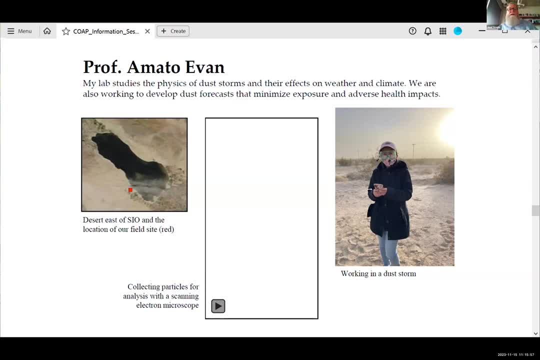 but there likely may be. Just give you a taste of what's going on in here that you could follow up with some of these professors, and there's more going on here than just that I've showed today. And, Kim, I don't know if you want to share something you're doing. 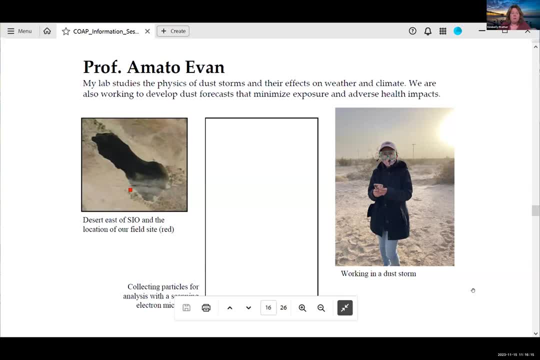 Yeah, I'm happy to. I was going to just sort of talk about sort of the crop, the work that's going on sort of across between different groups and across UC San Diego. Do you want to share your screen? Yeah, I can do that. 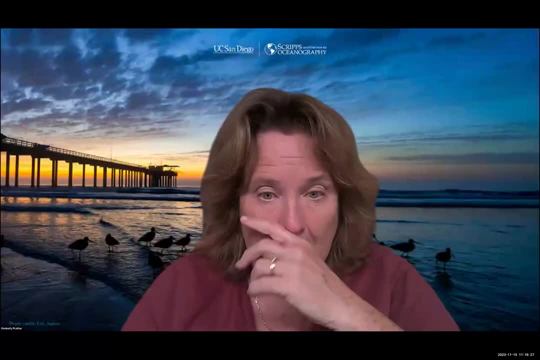 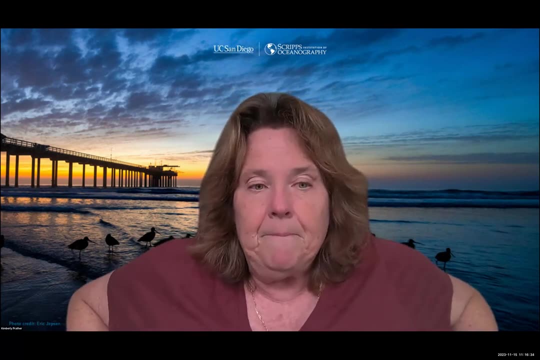 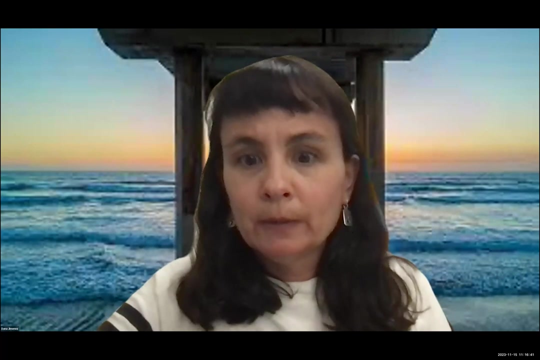 Okay, Okay, All right, can you see that? okay, Is that it? Can you see it? Not yet, Let me try again. Thank you, Let me try again. It didn't seem like it wanted to share. Okay, here we go. 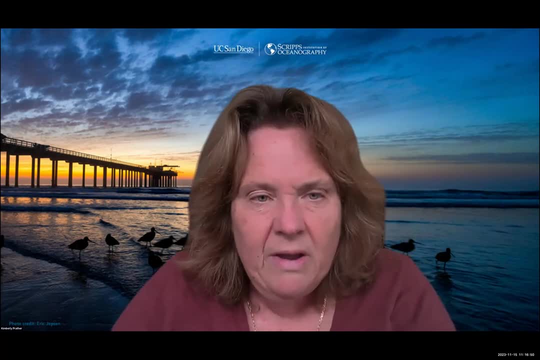 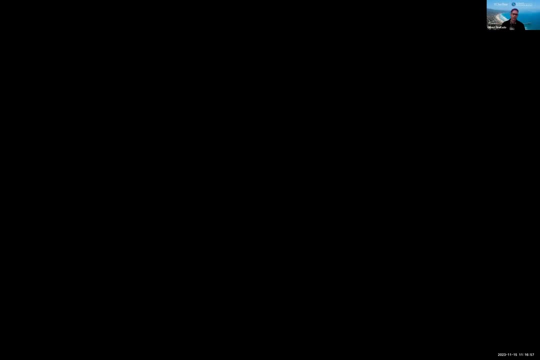 I see it. Okay, Let's try. Why is it being this? Okay, there we go Too much. How's that Is it there? Does that work, Okay, Thank you? Yeah, I'm just going to talk a little bit. 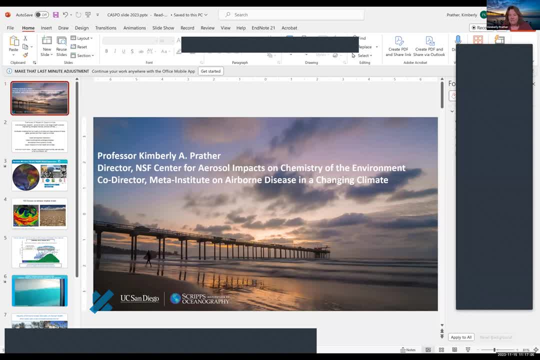 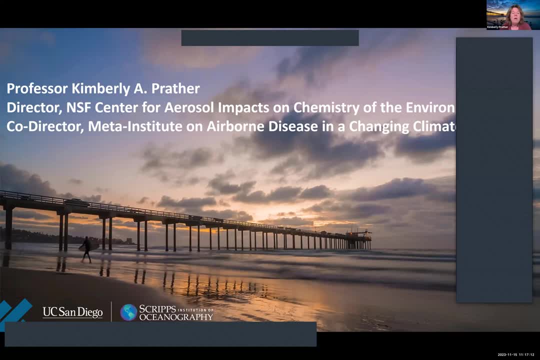 About some of the work. There's a lot of, you know. as you can see, there's a lot of research going on here And I'm just going to. I just think it's kind of exciting to see sort of all the work that's going on across Scripps and as well as across UC San Diego. 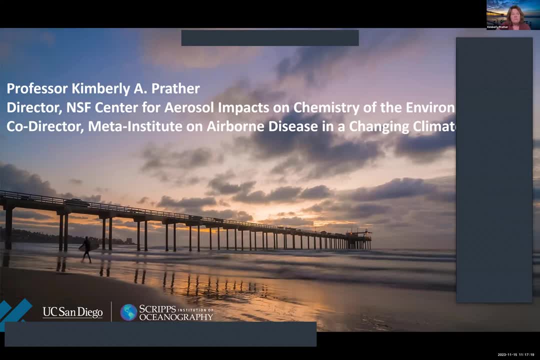 I'm a professor here at Scripps. I've been at Scripps for well at UC San Diego for 20 years. I direct the National Science Foundation Center, which brings together people across again, across Scripps, across the campus data science. 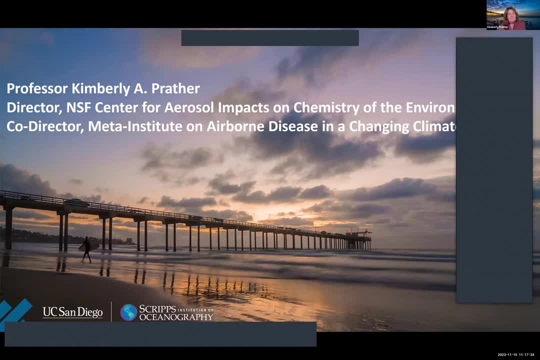 Oceanography, atmospheric chemistry, sort of microbiology. So it's a really exciting time here And the other. the other thing we've just launched is a new institute which is really looking at the effects of the ocean, Now not only sort of the effect on climate, but also the effect on human effects, on human health, which is becoming more and more prevalent. 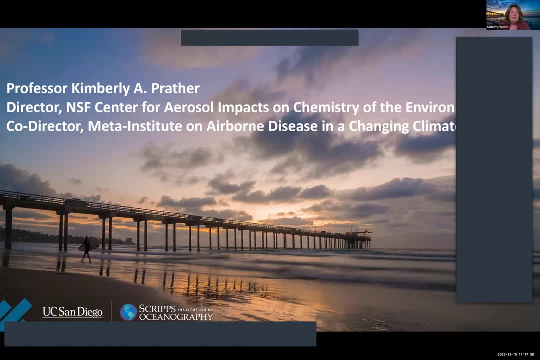 So, as I say, I'm just speaking sort of on behalf of a lot of other professors here at UC San Diego And I'm just going to talk a little bit about the work that's going on here. Okay, Thank you, Thank you. 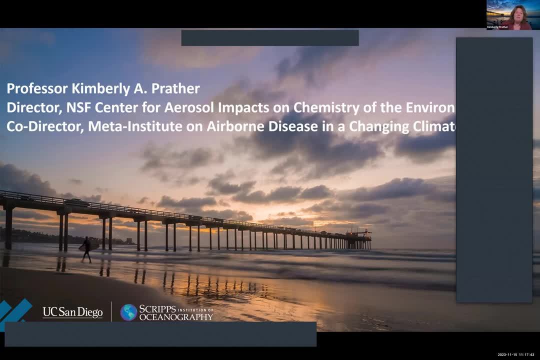 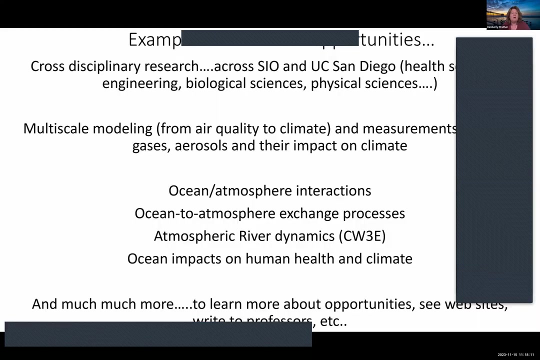 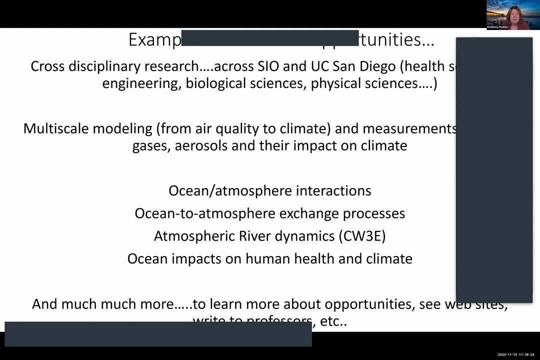 Yeah, Like one of those things that you said that we're microphone. Yeah, you know that we're trying to address. I mean, one of the things I think Scripps does well is train students to sort of tackle these large scale environmental problems, And so all the 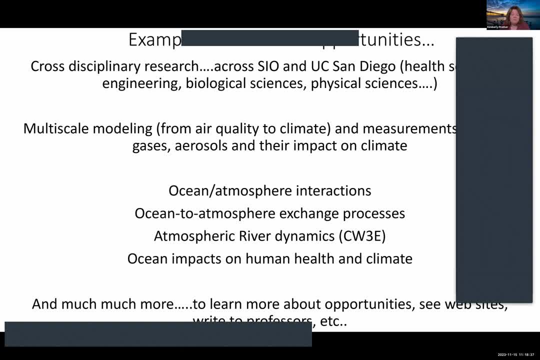 way from measurements to modeling. you know, and these are just a few examples of some of the areas where many of us are working together. I just want to make a pitch for you know, to learn more about these opportunities, I would encourage you to look at websites. I'd encourage you to reach out to 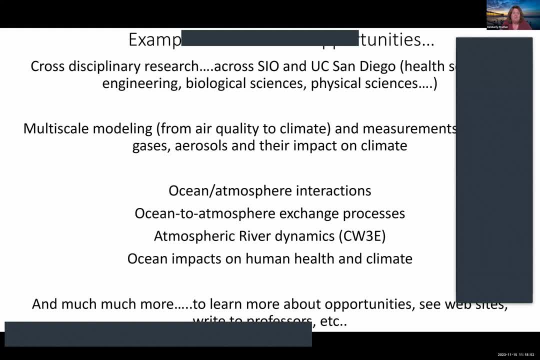 faculty. A little bit of advice: when you write to the faculty you know, talk about which aspects excite you the most. Make it as kind of a specific email is always something that catches our attention more, And we're happy to talk with any of you separately as you prepare your applications. 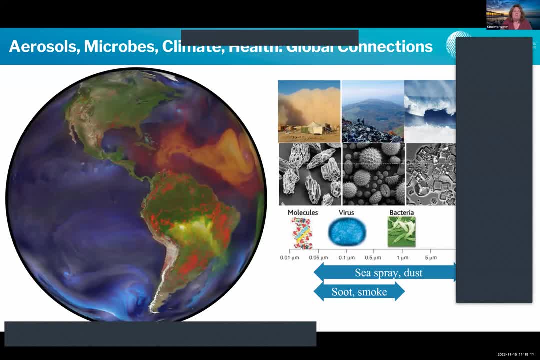 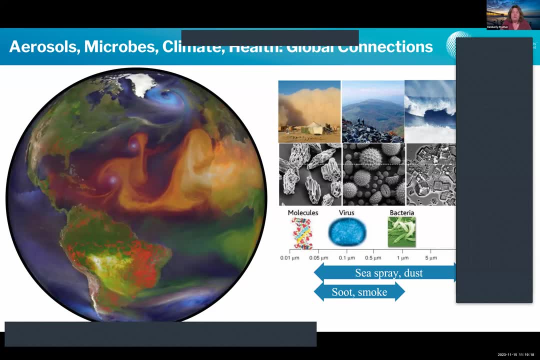 So I? this is a little bit of background on what I do. There's a lot of people here at Scripps that look at aerosols as well as gases in the atmosphere. I'm an aerosol person but do a lot on trace gases. 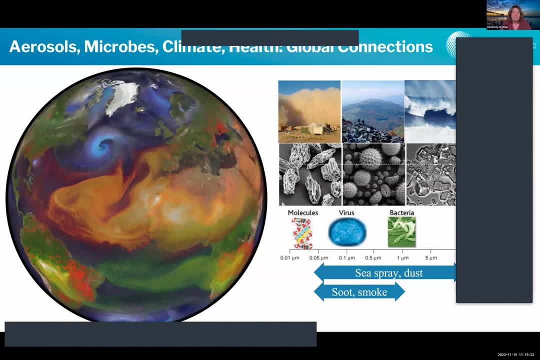 as well. So I'm a lot of people here at Scripps that look at aerosols as well as gases in the atmosphere as well, And I think most of you probably know what aerosols are. They've gotten a lot of attention through the pandemic But this just shows you know sort of how they interact. 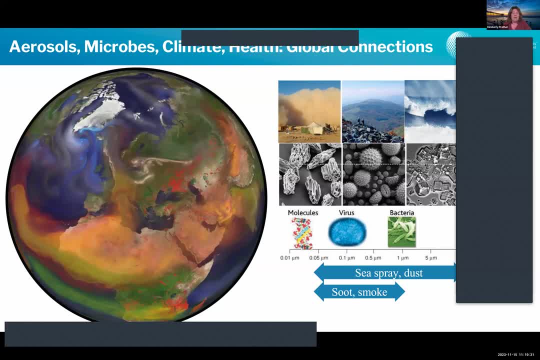 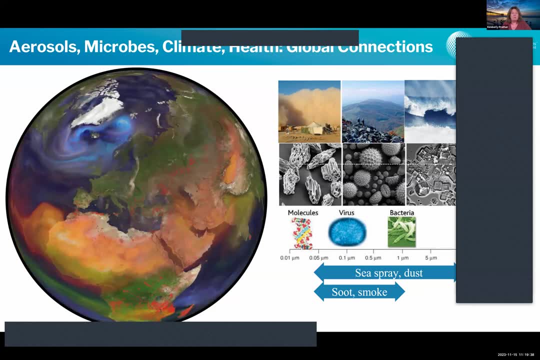 how they travel around the globe, how they affect our weather and climate. And again, there's a number of people here at Scripps that are working on problems related to aerosols from both a modeling and measuring measurement perspective- Another thing that people at Scripps are working- 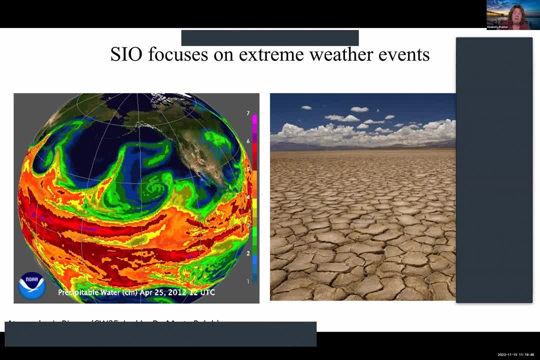 on, and there's a specific center that Marty Ralph runs- and many people are involved in it as well, called CW3E, The Center for Western Weather Water Extremes. I think I got those right, But basically as we, as our climate is changing, we're starting to see this pattern where we're getting either these: 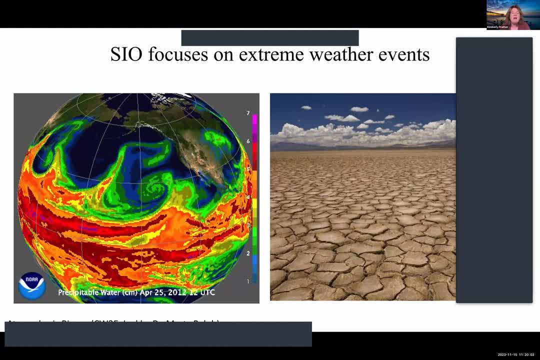 atmospheric rivers, which I think we're just on the verge of getting on right now, where we have lots of flooding, And there's, you know, Scripps is really a central place where that's being studied. But you either get too much water or not enough, And sort of we're getting this. 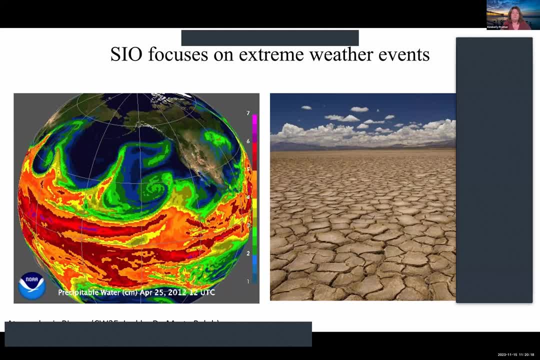 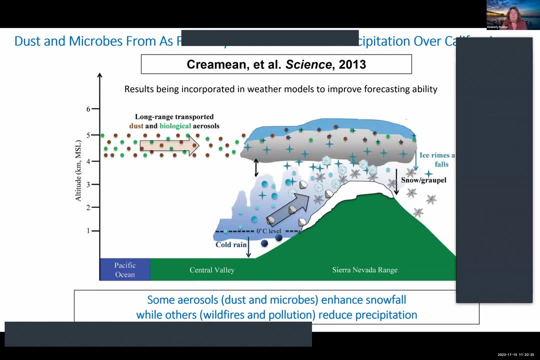 interesting split in how, basically as a result, as our climate is changing and so many of us are looking at that. This is a study we did with Marty Ralph's group years ago and we were able to show that dust in biological aerosols all the way from Africa changed the 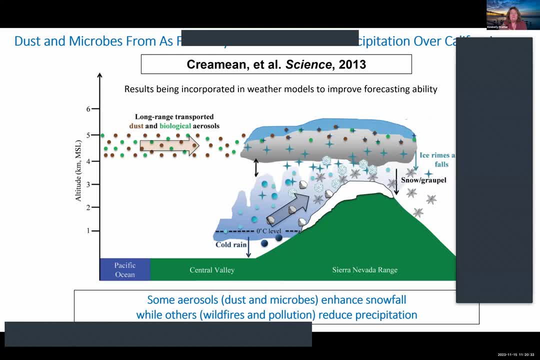 snowfall here in California, And so again, this is just an example of you know how you can combine atmospheric chemistry and weather and climate all in sort of one package and learn a lot about what's going on, And so this is one of our bigger discoveries. that was an exciting one. 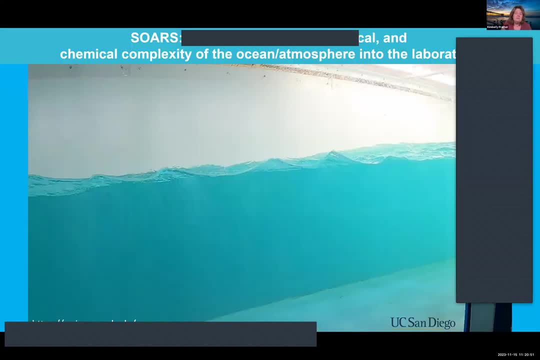 to make. I just want to also talk a little bit about the facilities. This is a new facility called SOURS. I'm just going to give a little snippet about it. but it's a global facility. It's only one of its kind. We can control the temperature of the water all the way to the point where we can make sea ice. 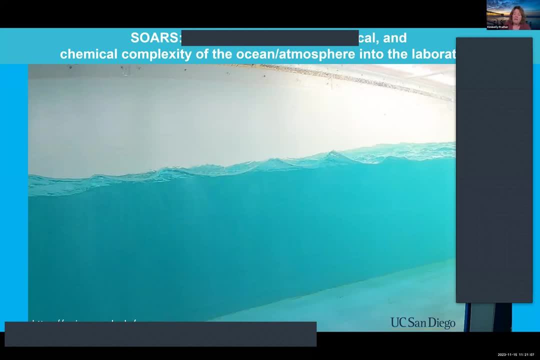 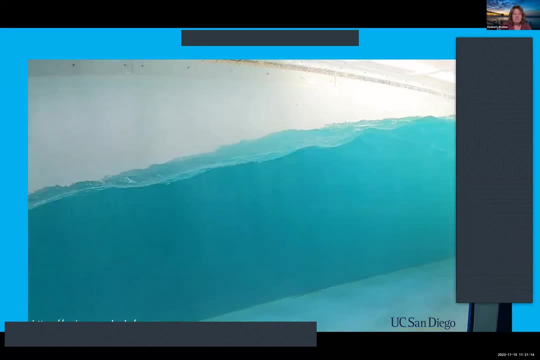 It's an integrated system with winds and waves and 36,000 gallons of seawater that we pump directly into the system. So let me just show you this. SOURS is an instrument. This is great. It produces the biology, the chemistry and the oceanography. 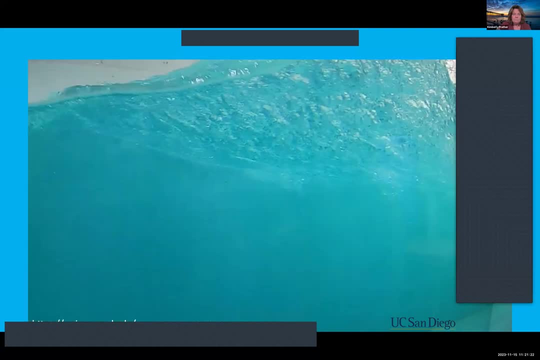 of the ocean And it's an instrument that can be used to control the temperature of the ocean. It's an instrument that can be used to control the temperature of the ocean. SOURS stands for the Scripps Ocean Atmosphere Research Simulator. It's an instrument funded by the National Science. 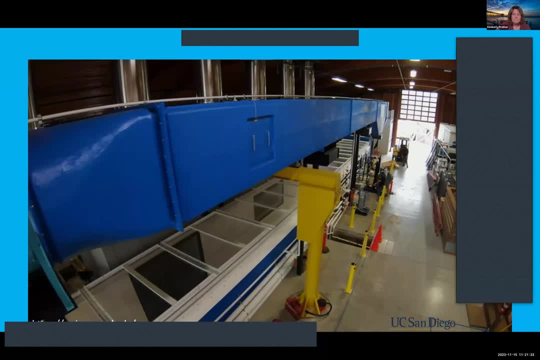 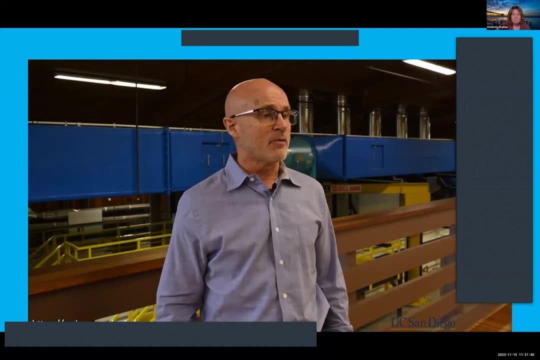 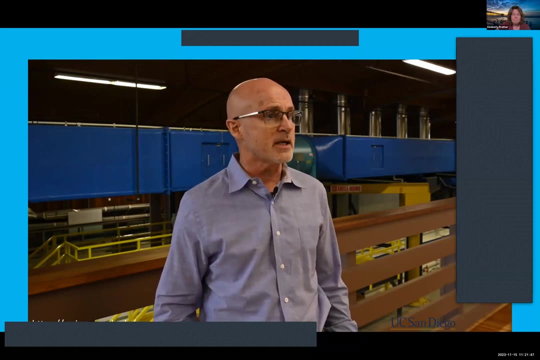 Foundation supported by UC San Diego. We've always known that the AC boundary is important. What we didn't understand was how the combination of biology and chemistry, and wind and waves were all working together to create this unique and special place that impacts weather. 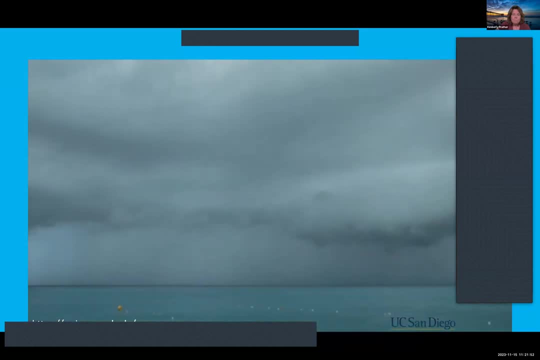 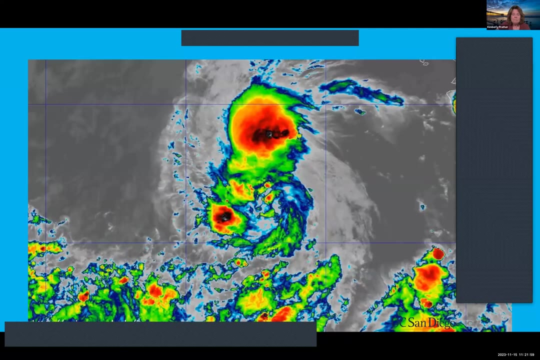 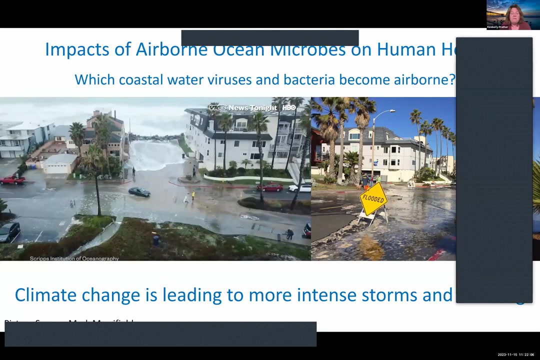 Now we're going to understand this complex connected system so that we can predict what future climate is going to look like and what future weather is going to look like. That gives you a little taste of that sort of the facilities that we have here, that you can, that every you know, that everyone has access to. 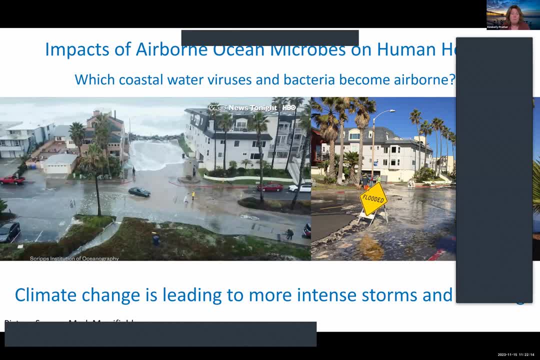 And, as I say, people from all over the world can come and work and basically use this, this facility. Another thing I just want to touch on. this is work That we did actually, picture provided by Mark Merrifield, who, I believe, is going to be talking about some of this. 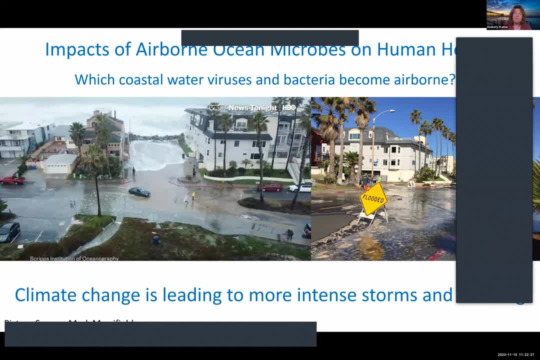 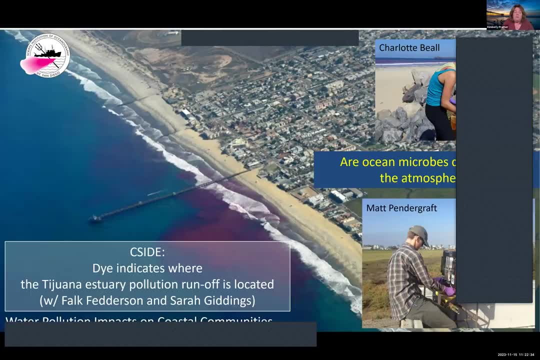 But it looks at flooding. that's local here, where we're getting billions of gallons of raw sewage down by the Mexican border, And so we work with Fault Federsen and Sara Giddings and many others, sort of one of the things that they do really well. 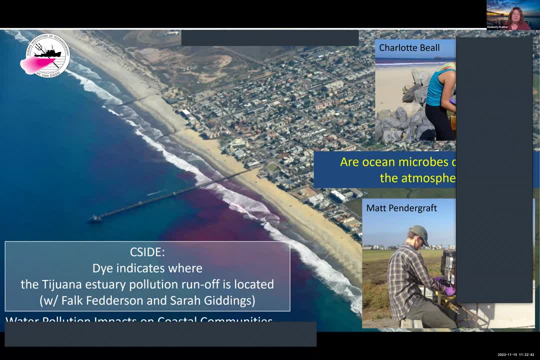 Is understanding ocean currents, And so one of the really powerful things that Scripps is that we have both people looking at the ocean as well as the atmosphere. But now we're really starting to work together to look at the combination because, as we know, they're connected, but a lot of times people will look at one or the 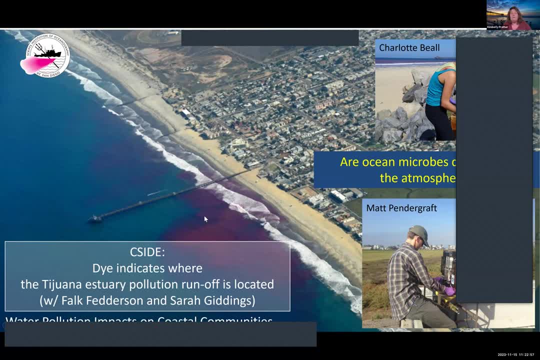 other um. so we piggybacked on this early study where they put dye in the ocean. they've done this now twice and you can look at the currents, and those near shore currents are the ones that are really hard to map out. but the idea was to look at at sort of how far the pollution went and how 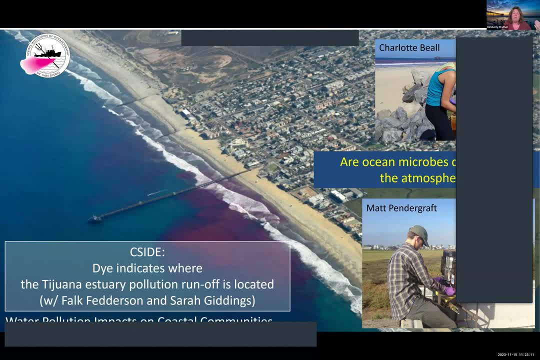 it impacted people who went to the beach or swimmers. we came along with air samplers. these are a couple of my graduate students um matt in charlotte that have both graduated now, and we looked at how this waterborne pollution impacts the air, and so one of the really exciting things. 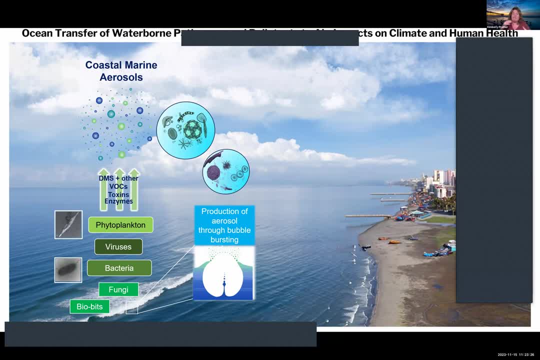 i think that we're that that is going on here is sort of thinking about this connection between the ocean and the atmosphere. this is work from the center, the nsf center- that i ran for 13 years called case, and it really looks at what gets out of the ocean all the way, from all the microbes. 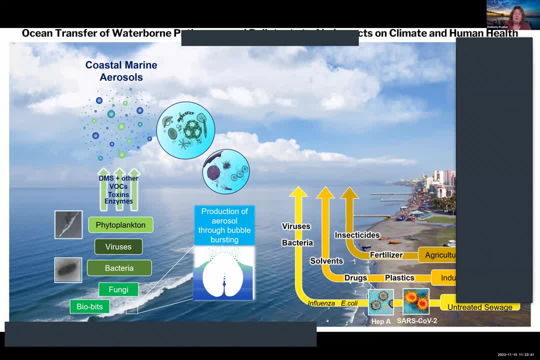 um to the gases that get out. but now we're starting to really think about in this region and other regions of the world: what about the human? what are humans doing to coastal environment, and how is that affecting our air quality and climate? so this is a brand new project that has 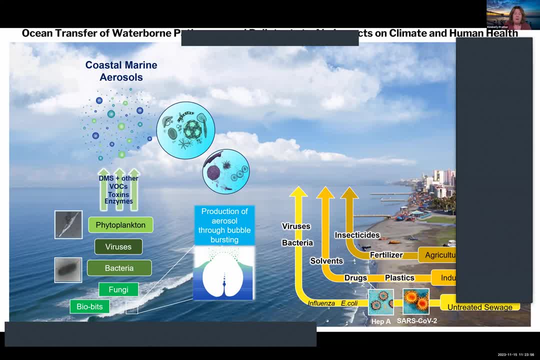 created quite a bit of interest. um, and there's again a number of researchers here at scripts that are working on this project, and so one big question is: is this a way that people can get exposed to pathogens and pollution? answers: yes, but we're trying to understand this better now. 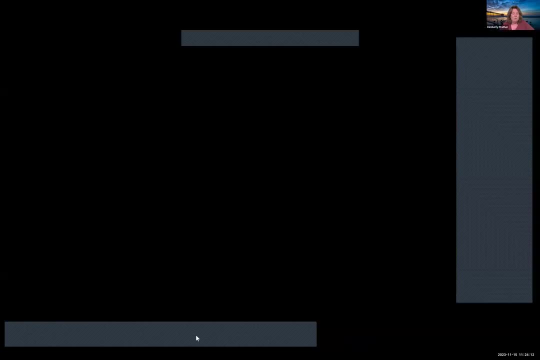 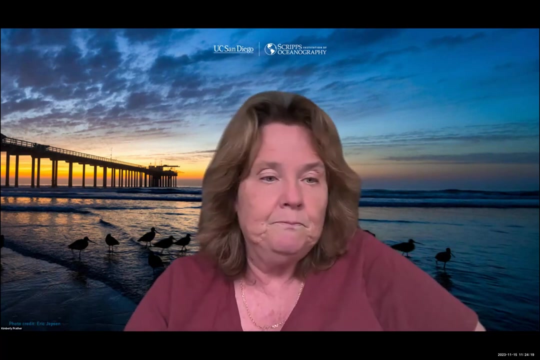 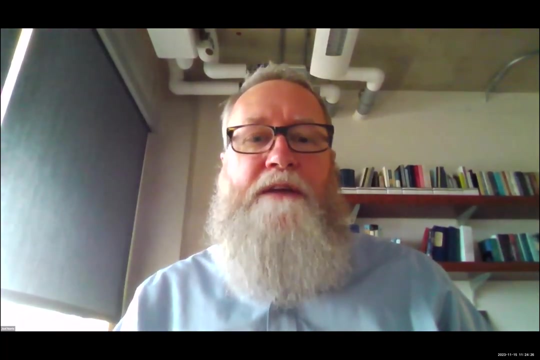 so i think that's it. i'm going to stop there. i just wanted to give you a little bit of a taste of what we're working on and i'm joel, i'll hand it back to you. thanks, kim, that was really great, showing that um all the various connections that come together. 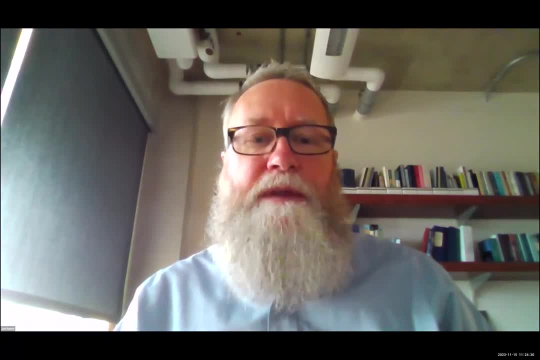 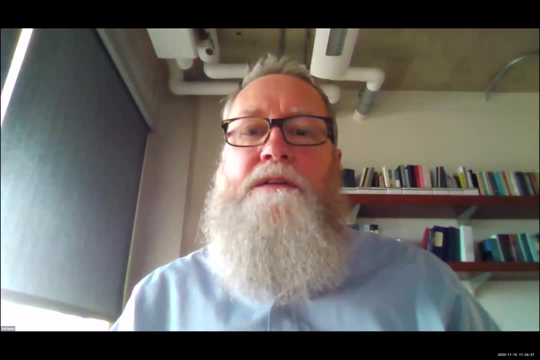 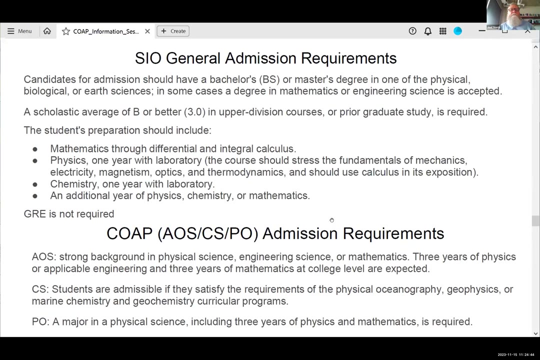 with all the different research directions people are doing to put something bigger than the sum is bigger than just parts, and i think let me share my screen again. i'll go back to the um. okay, here's just a list of the general admission requirements, um. i think this is on the website. this is so that um students are prepared to succeed in our courses in the first year and have a good foundation for their future research. 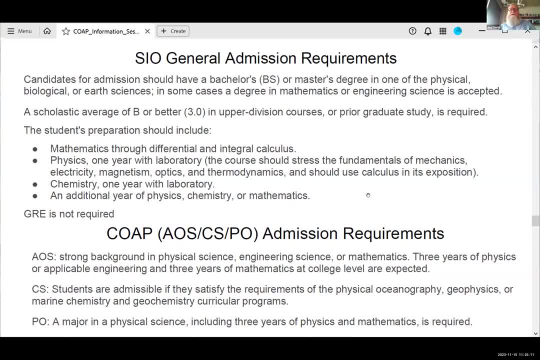 and- and often it helps to have more course background in physics or math or chemistry, depending upon your research area- then is than is here, so more is helpful. but this is the basic requirements and they differ between the three curricular groups because the three curricular groups have slightly different of. 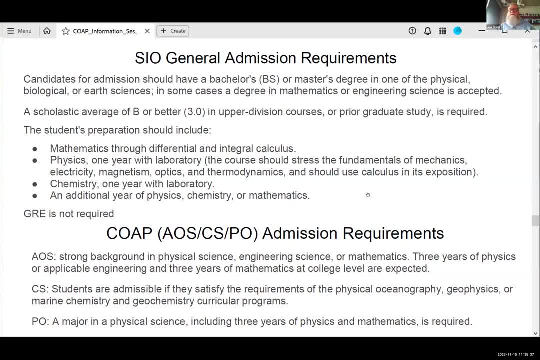 they have different first-year courses and different areas of research focus and I think maybe specific questions about the admissions requirements for curricular groups can be handled in the breakout sessions. but maybe if there's a general questions about the requirements- I don't know if there's any- 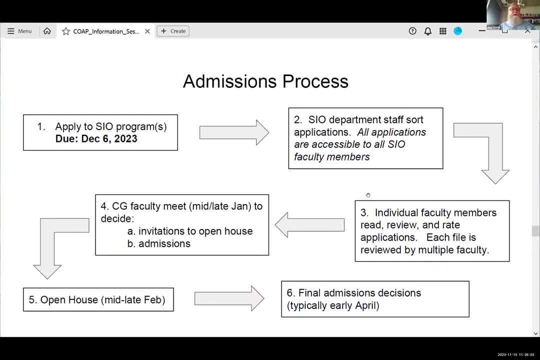 The process is here. I think this year the applications are due on December 6th and then they're going to be. every application is going to be reviewed by multiple faculty, depending upon the format, and then they're going to be reviewed by the faculty. 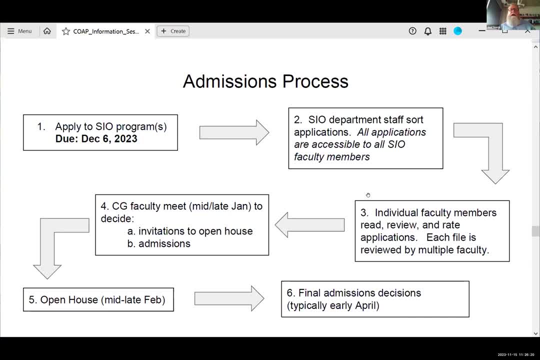 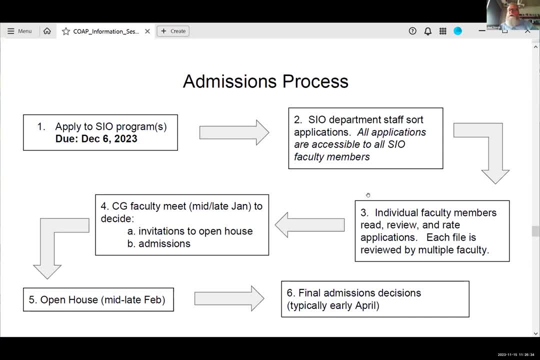 meet in mid to late January to decide preliminary admissions of students and then also invitations to come to our open house and meet faculty in person, which I think think will be- I don't know the exact date- Yeah, Sometime in February. So I think a couple of 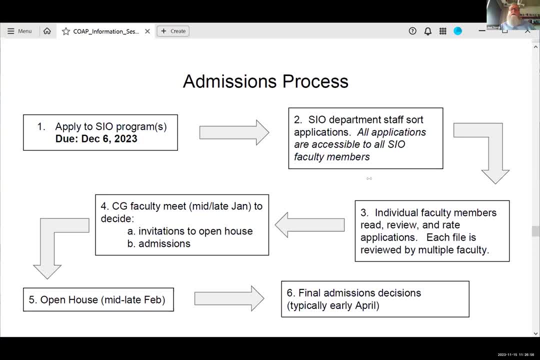 questions came up in chat. Joel, it's February 29th and March 1st for open house. Okay, Let's see, Um? okay, So I think, um, we have a couple of questions, maybe some that can be handled in the. 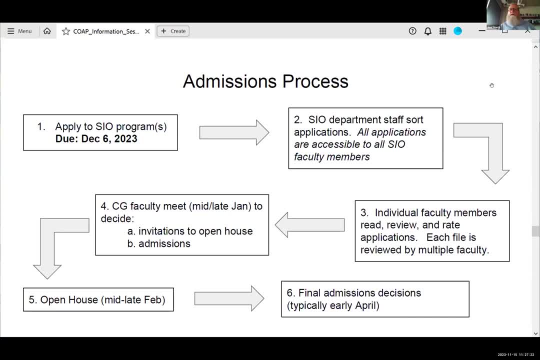 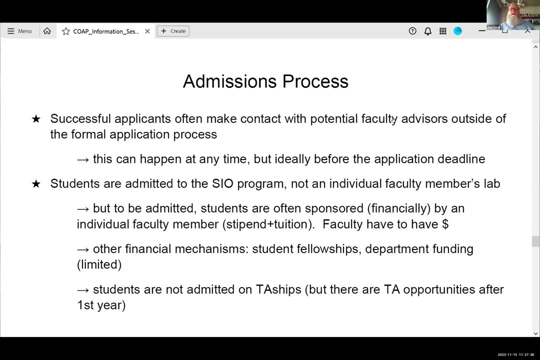 um, in the uh breakout sessions, Um, and then, uh, final admissions decisions we made in early April. Okay, Okay Now, um, we have both PhD and master's students here. One thing, um, it would be good. 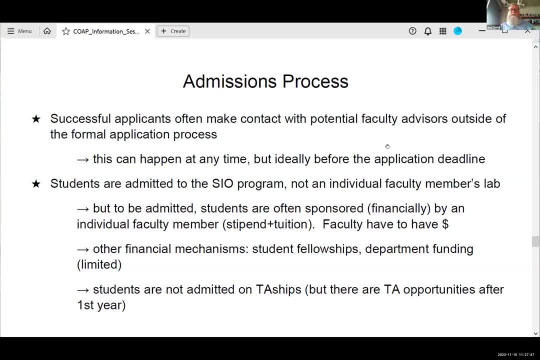 to make clear is that there are some, some um fields of of, uh, science or engineering where you do a master's first and then a PhD, but that's not the way we do things here. So if you are interested in doing a PhD, make sure you apply to the PhD program. It's not necessary to have a 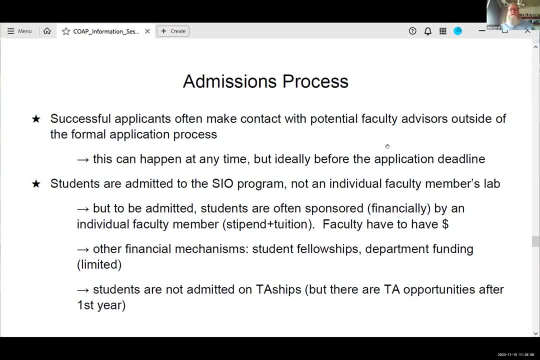 master's first Um and um. also it's useful um to talk to potential faculty advisors ahead of time to see if you- if they look like they're working in an area where you have some research interest- maybe like to do a project or something related to that, to contact various faculty You can see research. 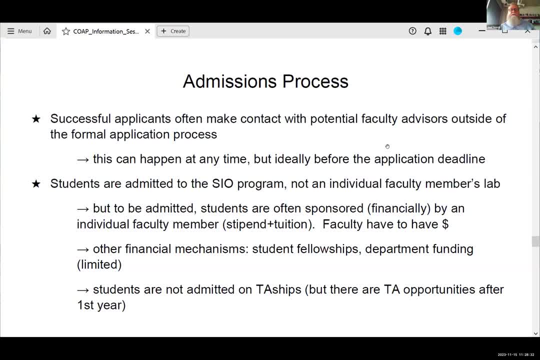 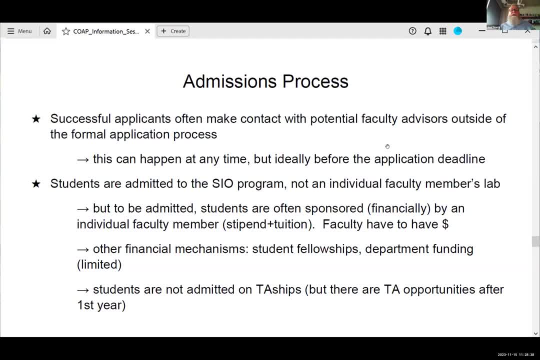 and make an email And, as as uh, as as uh Kim Prather said, you could, um, you know, explain, like what your potential interest is and, and you know, ask some questions about what's going on. 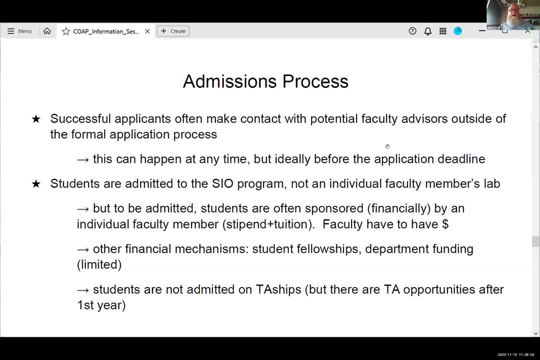 in in in the lab, And so all students are admitted into the program. They're not admitted into uh individual faculty members groups, but we have to. most students are going to be supported on research funding and a graduate research program And so um you can see um. 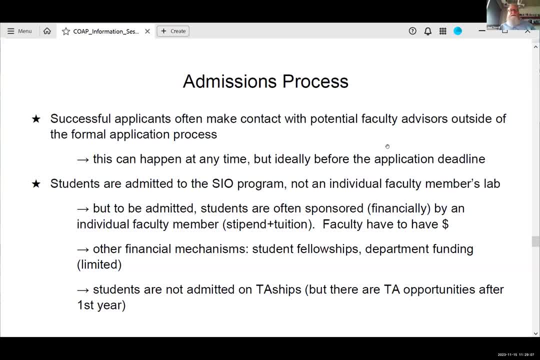 the graduate research, uh, uh, uh, uh uh, assistantship, And so, um, we need to make sure that the, the, that the funding is there to admit a student into that, um, into that area. Now there are a few student fellowships and department. that's pretty limited If 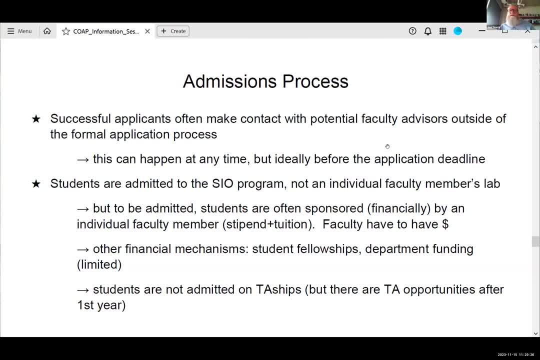 you come with your own fellowship, then you have a lot more uh freedom, Uh. but most students are going to be supported by um research grants. So that's why it's good to talk with faculty to see if they have funding available in an area you'd like to, you know. 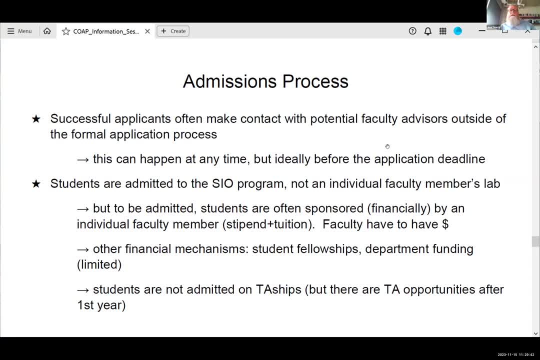 or a person you'd like to work with, And so, um, we, we do have teaching assistantship and sometimes master students get a TA- uh uh TA ship during their first year to help support them, but that's not guaranteed that you can get a TA ship, Um, for PhD students, they don't TA in the first year, but they may be able to get a TA in the first year. Um, so that's, that's, that's, that's, that's, that's, that's where you won't be able to TA after the first year. 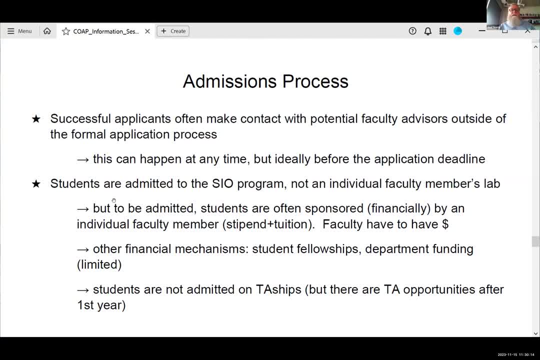 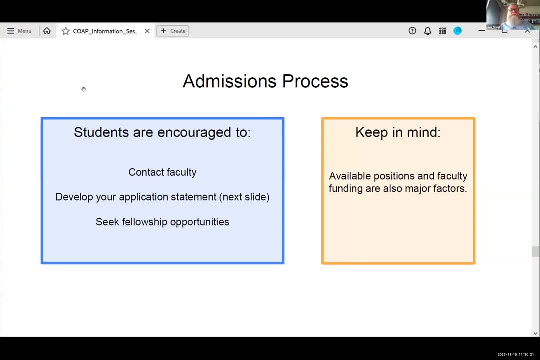 Okay, And so, um, we encourage you to contact faculty- I'll talk about uh- state your application statements in the next slide- and also seek fellowship opportunities, because if you have your own fellowship, that gives you a lot more flexibility. 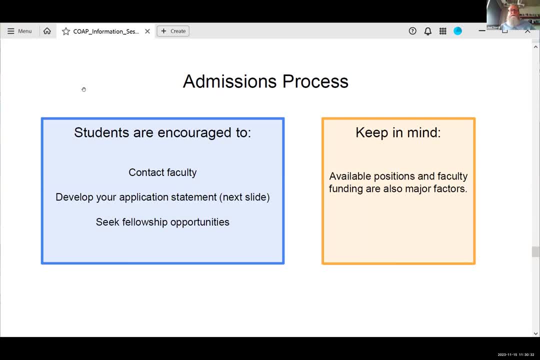 in this type of work you're going to you, you can do the type of research, Whereas If you're supported on a grant, then your research project has to be related to the focus area of that grant, And so what positions are open and what faculty have funding do play a major role in student admissions. 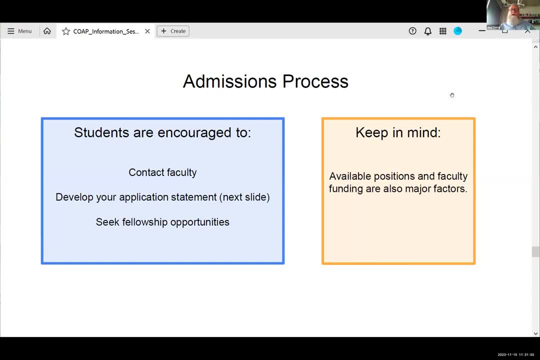 And so also we're looking for students to have a project or a research area they'd like to work on. that is something that we can. there's faculty member who can support and mentor that, and also that there's funding available to support that student. 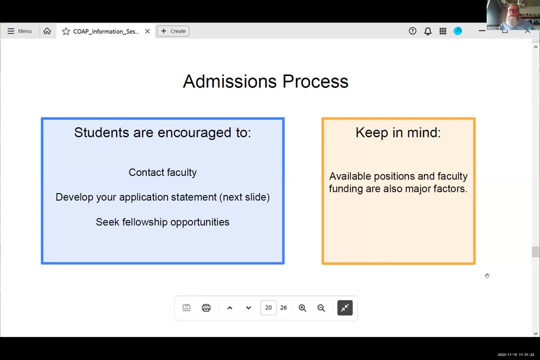 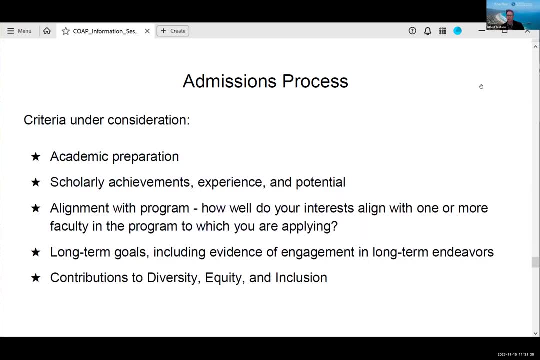 Okay, so, Gilbert, go ahead and tell me if there's any questions I should answer here in this session. Okay, It doesn't look like it. Nothing come up yet. Okay, Okay, so for the admissions process. what? what do we look at? 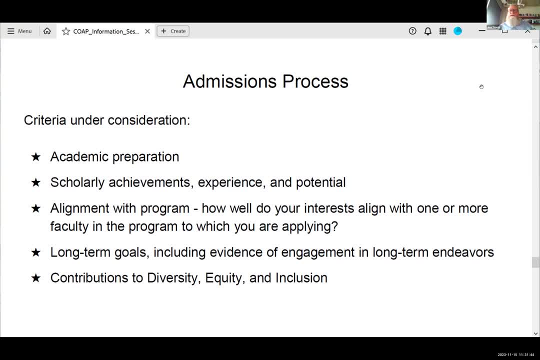 One is your academic preparation. we want to make sure the students who we admit will be successful in the first year coursework and have a good foundation for the research projects, And so we also look at scholarly achievements, experience, potential And, and it's not it so it does help to have, you know, undergraduate research experience, but we also recognize not everyone has had the same opportunities. 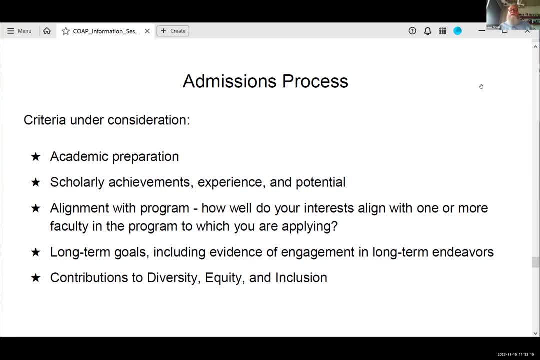 So I think it's important to see not you know all the things that you have done, but also you know how you've made use of the opportunities that you've had. And another big factor here is the alignment with the program. 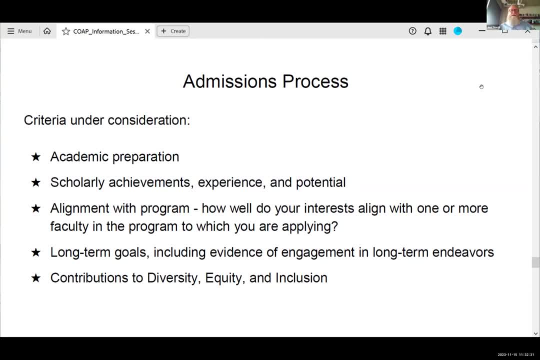 And so if you have research, Research interests that don't really fit in with any faculty member, it's going to be difficult to admit you, because we don't want to admit a student who can't be mentored in the research interests that they have. 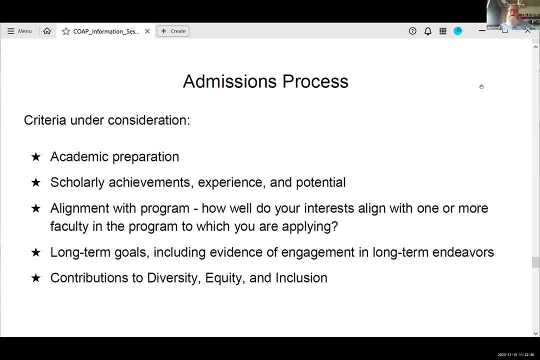 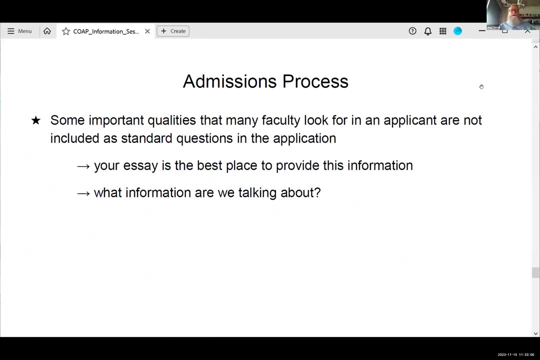 And so that's why it's good to look at the faculty here and contact them ahead of time to see if there's going to be alignment, And we also look at long term goals and contributions to diversity. So there's going to be a statement of purpose or out, exactly what it's called now, and this is not like. 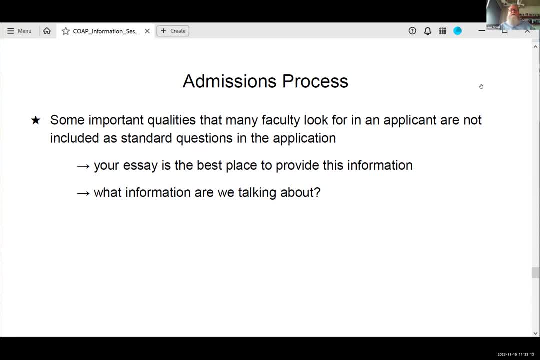 undergraduate applications be until undergraduate college. for this thing we're really looking for What you're interested in doing, what's your research interests and how Coming to scripts can help further that, And what your background is and how that fits in, and so this is really a place for us to see like to really tell us about yourself and what you're looking to get out of, why you want to do a PhD and how you see that could happen here at scripts. 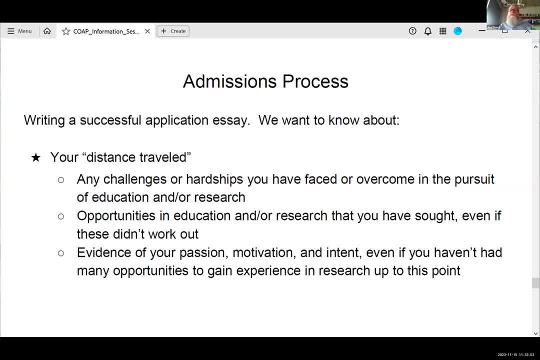 And so you can talk about. you know challenges or hardships, and all of us have had that. And so you can talk about. you know challenges or hardships, And all of us have had that And all of us have had that. and so no one you know comes here with a perfect record and 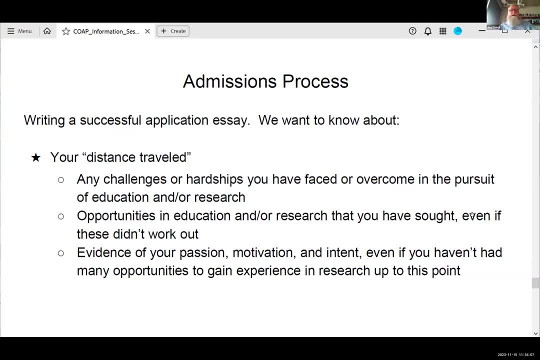 And you know how you've made use of opportunities you've had And you know. and also motivation, and we don't expect people to know ahead of time exactly what research they want to do. sometimes they come here and discover new things that they were not aware of. but we'd like to. we like to see students who have some idea. And so no one you know comes here with a perfect record and And you know, and also motivation, and we don't expect people to know ahead of time exactly what research they want to do. sometimes they come here and discover new things that they were not aware of. but we'd like to. we like to see students who have some idea. And you know, and also motivation, and we don't expect people to know ahead of time exactly what research they want to do. sometimes they come here and discover new things that they were not aware of. but we'd like to. we like to see students who have some idea. And you know, and also motivation, and we don't expect people to know ahead of time exactly what research they want to do. sometimes they come here and discover new things that they were not aware of. but we'd like to. we like to see students who have some idea. 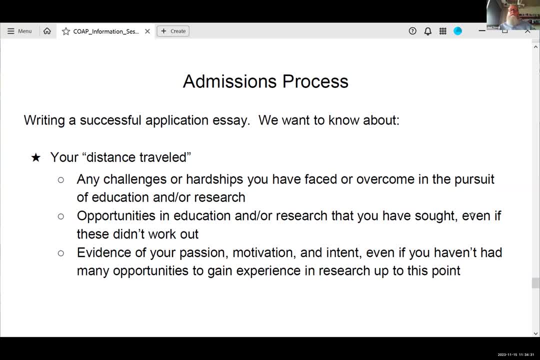 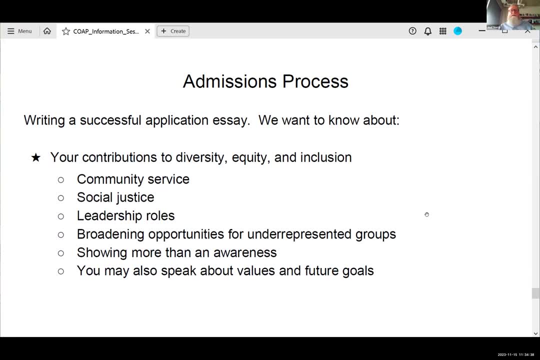 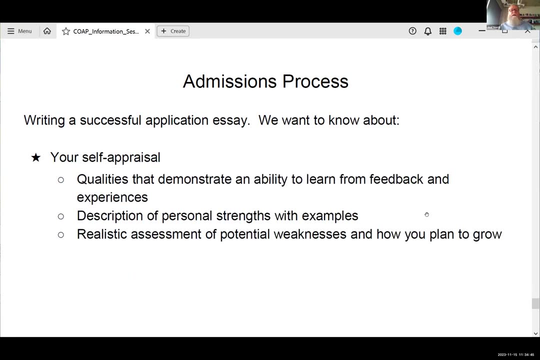 and how that might fit in with our program here, And so the contributions to diversity, equity and inclusion, And also, you know, a self-appraisal. So this is also an opportunity you know to share about yourself and how you've made use of opportunities. 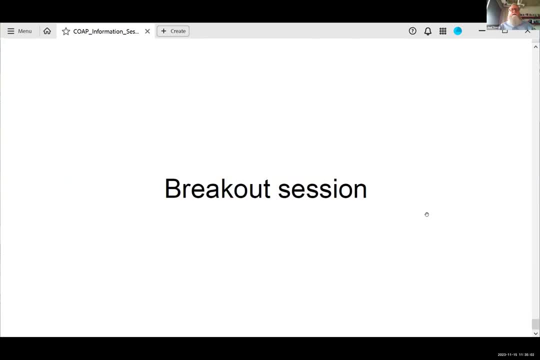 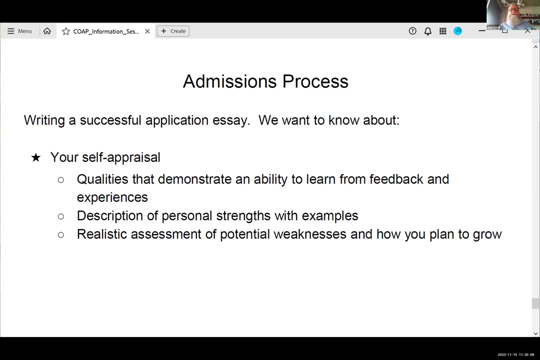 and challenges you faced, And I think that comes to the end of the general admissions information. Are there any questions? I can answer Gilbert. Yeah, there's a general question about the issue of funding. Is it appropriate to discuss that when reaching out to? 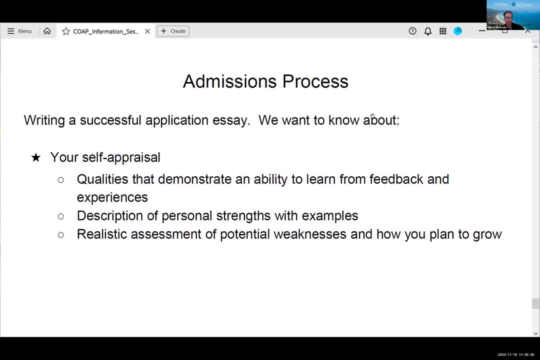 particularly Okay. yeah, where is this question? It's in the chat. So when reaching out to prospective advisors, is it appropriate to ask if there is funding to take on a student? Yeah, I think that's quite appropriate, because if there's not funding to take on a student that year? 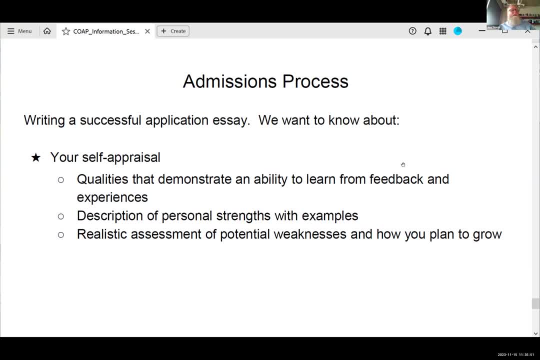 you know, if you don't have a fellowship, if there's not some alternative, I mean that would be something that would have to be worked out with the advisor. But basically, every student that gets admitted, we want to have identified funding for that student. 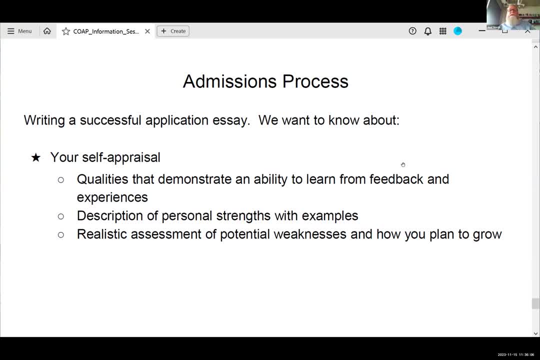 one way or another. So that is something appropriate: to ask advisors either if they have funding available or if there's something you can do to put together funding. And there's a couple other questions, but they were more kind of administrative So I was answering them in the chat. 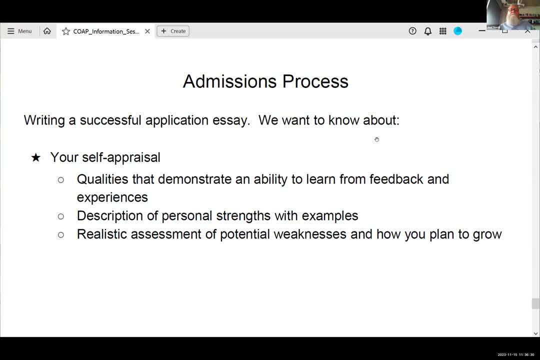 Okay, Let's see. Should I glance through some of the chat here, Or? I guess people could also raise hands. Yes, If that could be seen. Okay, There's a question about: are integrated masters of science, masters recognized, Although I don't know if that's relevant to admission. 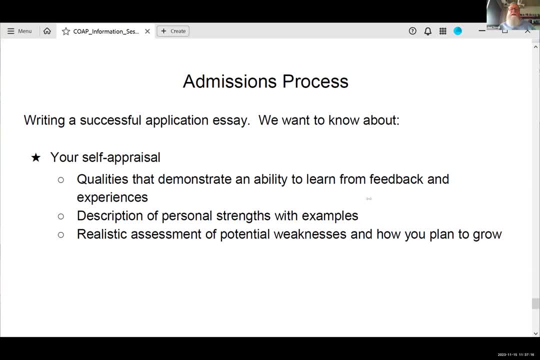 I guess that. oh, I guess, Gilbert, you answered that. You answered it in the other part in the chat. sorry, Okay, DEI part. Yeah, that's what I was going to say. I don't know if, like, I guess, I'm probably not the best person. 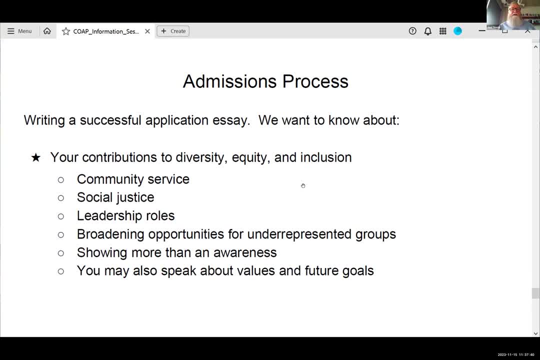 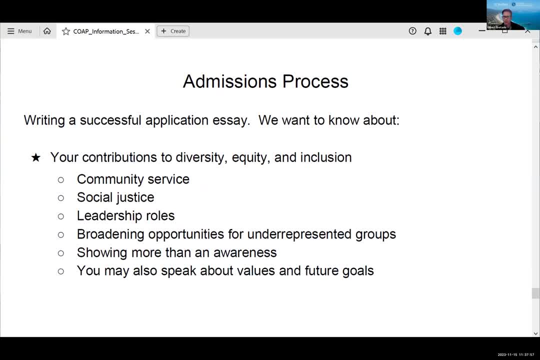 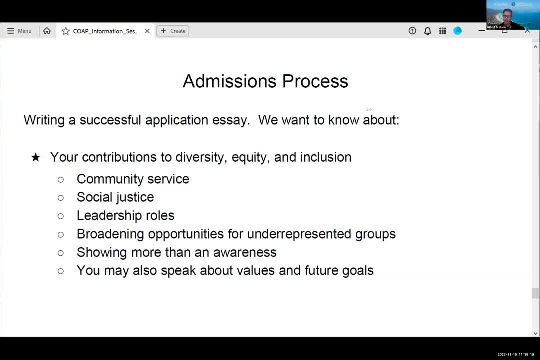 Okay, So you know, at this point in time we had that additional question about funding international students. So we generally we admit California residents, non-residents and international students across the program. your funding, the funding guarantee that you receive. 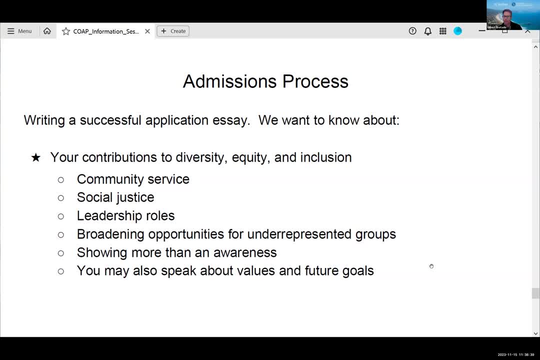 will cover all the Scout tuition and fees. So if you're an international student, that includes the non-resident fees. If you're a US citizen or permanent resident, your financial guarantee would include the non-resident fees for that first year i mentioned. 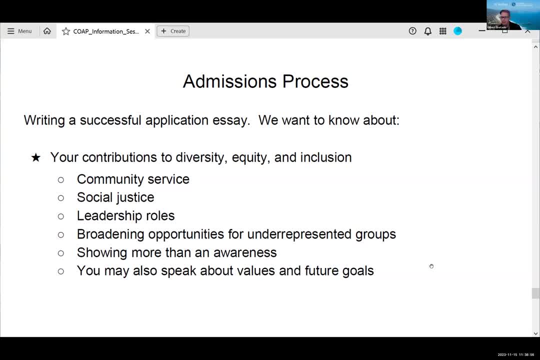 in the chat. for those students, they are required to become california residents for tuition purposes at the end of their first year. but, um, just generally speaking, we, we don't differentiate between applicants, so other departments might have a focus on just admitting california residents because of the the cost associated with it within scripts. we, we don't take that into consideration. 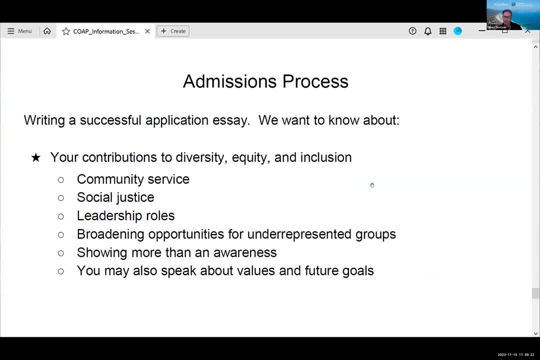 when admitting students. um, and as a as a admitted student, your financial guarantee will cover whatever applicable tuition and fees are associated with your, your residency. yeah, i think a question came up: it's not necessary to have a master's degree already, just a bachelor's degree. okay, i think there's. i think maybe a question about physics backgrounds like. a question like: 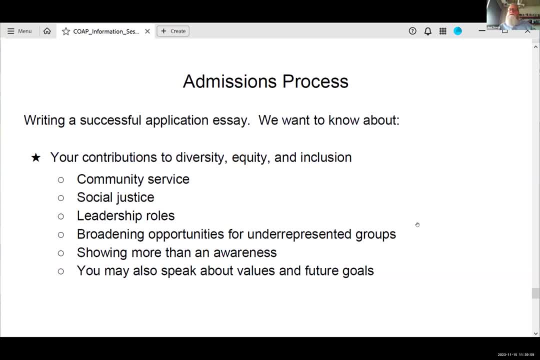 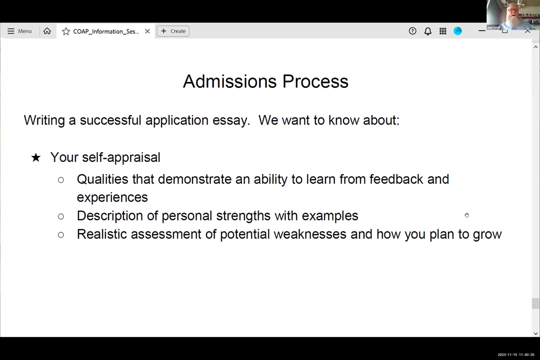 don't have enough. i think maybe that'd be better off than break the breakout sessions, because that may be specific for the curricular groups, like background physics courses. um, uh, yeah, so are there any more? yeah, gilbert, should we go to breakout sessions, or or i don't know. yeah, i've come to the end of of my part here. 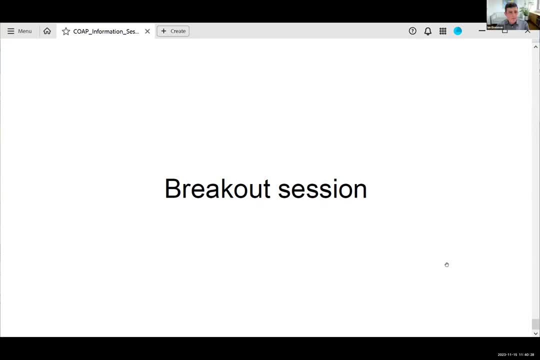 yeah, i'll go ahead and open up the breakout rooms. there's a question? yeah, i think you're going to say what i was going to say: go ahead. i wonder if you want to respond about a few waivers. the waivers: yeah, so unfortunately, fee waivers um ucst only provides fee waivers to. 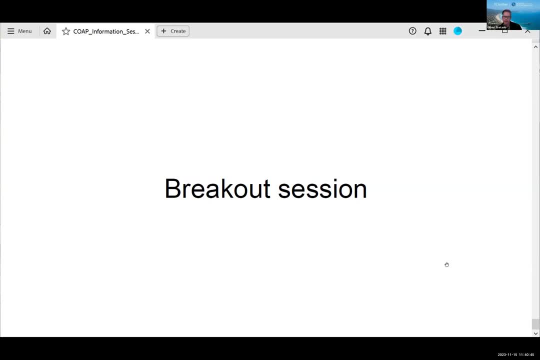 domestic students, so international students are not eligible for fee waivers. all right, so i went ahead and opened the breakout rooms. they are titled based on the curricular groups, so applied ocean science, climate science and physical oceanography, and so whatever group you are most interested in, you should be able to to just go ahead and join that room on your own. 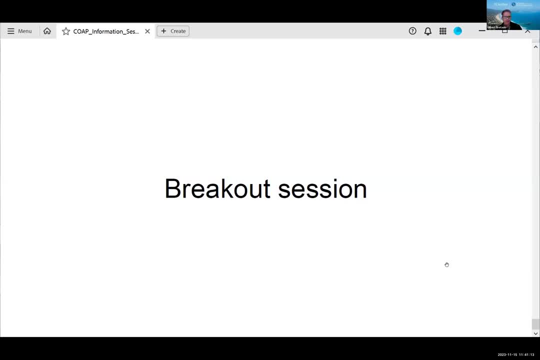 if you're not, please, please, let me know. um, and, like i said, if you want to jump in to multiple rooms, you're welcome to do so. and then, joel, did you want us to convene back in the main room at the end or just end at the end of the breakout room session? i, i think we should probably end at the breakout. 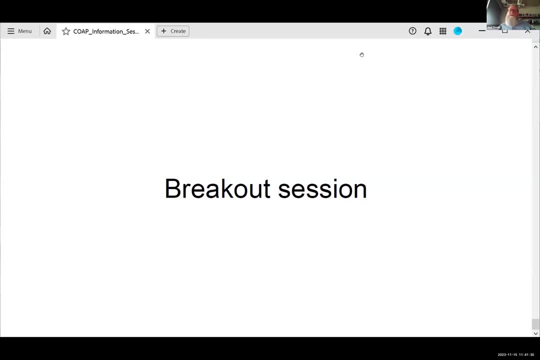 because i don't know if we're going to end the breakout sessions going to end at the same time. so, um, would there be a reason to come back into the main group? um, i don't think so. if you covered all your slides, um, yeah, so maybe we can just aim to close. 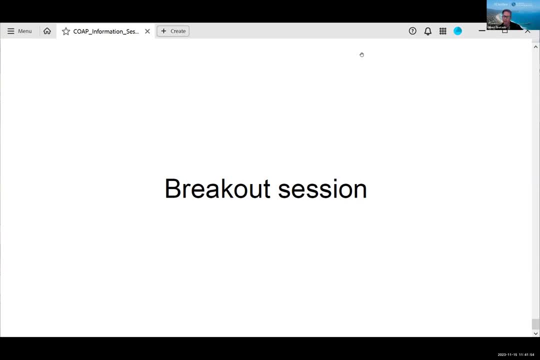 the breakout rooms about 12 and if you know people still have questions, they can continue on, but otherwise we're just in things within the breakout rooms at around noon. okay, well, that be enough time. i guess 20 minutes, i guess it's just for questions then. yeah, yeah, and i will keep them open, so so, 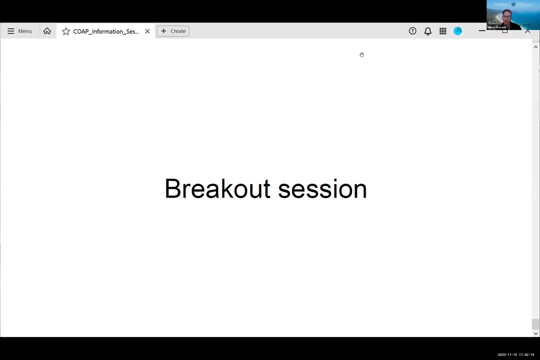 folks are welcome to stay as long as they are available. uh, i'll see you guys there for the next 12 minutes and then we'll get back to you guys this morning, as long as they want. just to give everyone kind of an idea on the format for the rest of the day. 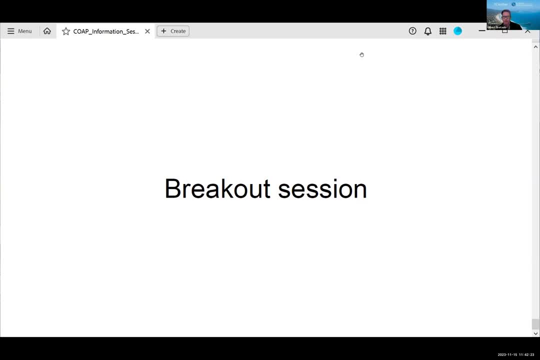 Okay, And Dana and I will hang out in the main room, so if anyone has any technical issues, feel free to pop back into the main room or send us a message. Do I have any more formal role here? This is my first year doing it. 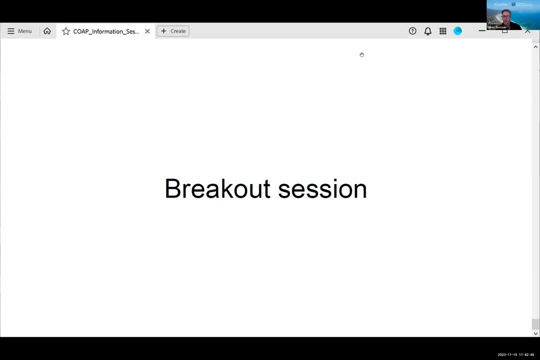 I think you covered everything as program director, so thank you. Okay, I guess I could go to climate science. That's what I'm most familiar with. I mean, do I, is it expected I show up in a breakout rooms? I don't know if I could really answer. 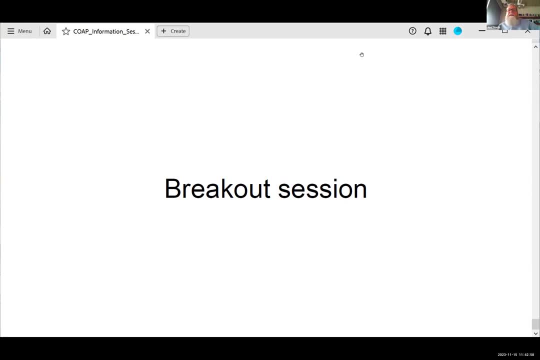 any better questions? any questions any better than the than the curricular group directors? Yeah, I think Nick is taking the lead on that. You're welcome to join if you'd like. I think, yeah, you'd probably answer questions.